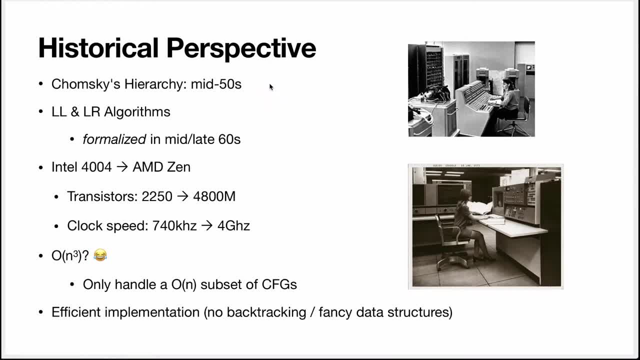 of languages and grammars in the mid-50s. The algorithm we're going to see, LL and LR- were formalized in the mid or late 60s And I put formalized in italics because probably people at the time were writing parsers by hand that were doing similar things Maybe. 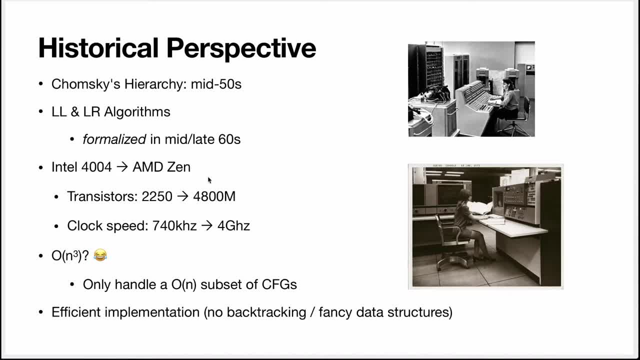 not totally similar, but fairly similar. At the time, computers looked something like this: So this is a computer from 50s And this is a computer from 71. It's an IBM mainframe. Actually, those are computers that use processors. 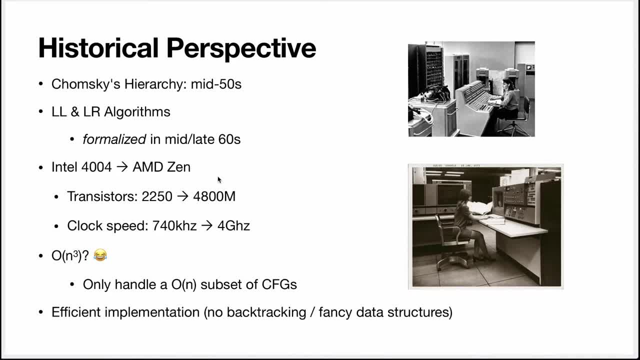 but not microprocessors. Those were also introduced in the early 70s And the first microprocessor was the Intel 404.. So I've compared the 404 with the AMD Zen, which is a recent processor, And so you see that the 404 has about 2,000 transistors and the Zen 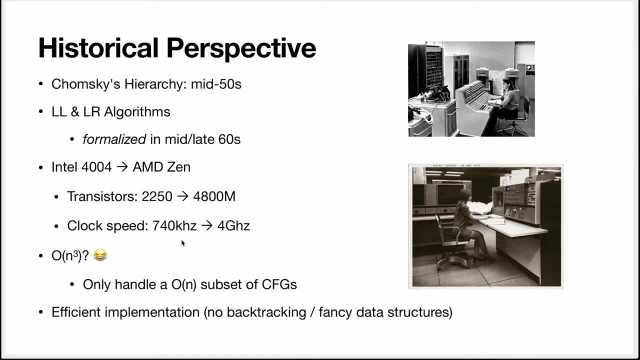 has almost 5,000 million transistors. The clock speed also went up more than four times, So it's quite a leap. There's a 8 million performance. It's probably more complicated than that, But you can imagine the scale of things. 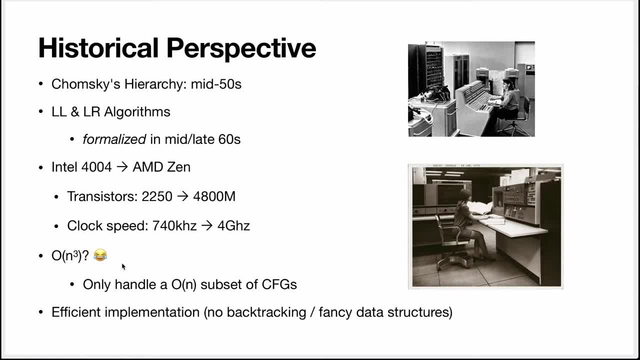 So at the time the idea to parse all CFGs in O n cubed was completely laughable. It's way too slow. The solution, then, is to only handle the O? n subset of context-free grammars, And for programming languages that is very practical. You can almost always come up with a grammar. 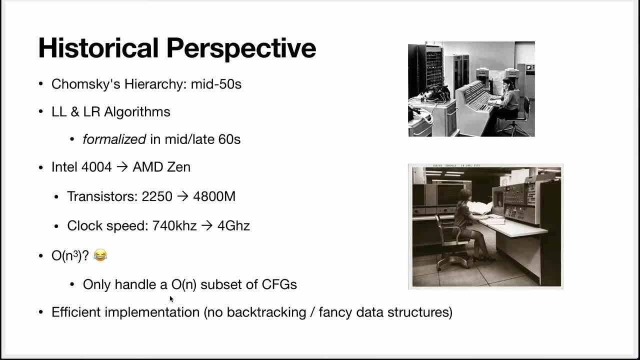 for a language that is linear in practice, For linguistics which, remember, Chomsky is a linguist. He's not a linguist, He's not a computer scientist. For linguistics, the O n cubed parsing algorithm might be practical. 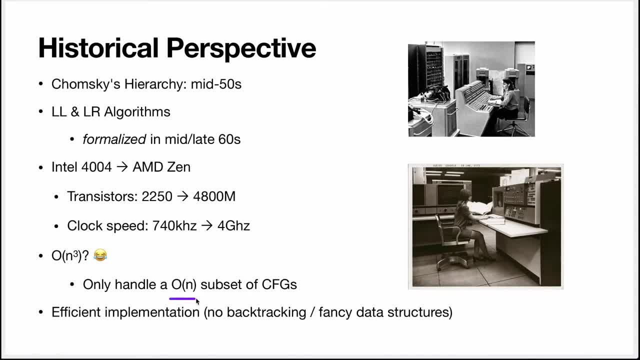 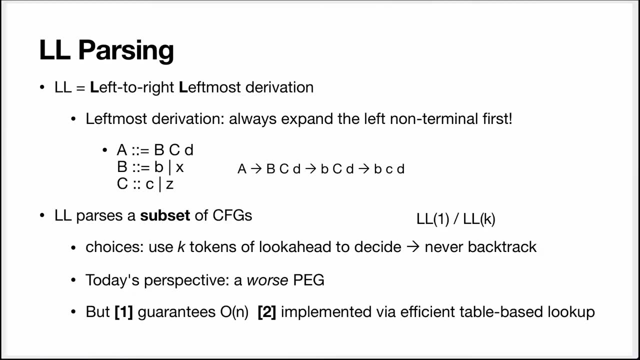 Not only do we want something that is theoretically effective, in the sense there is a linear bound, but we also want a practically efficient implementation. So that means mostly using efficient data structures and, in particular, direct array access, because it's very fast, and no backtracking. 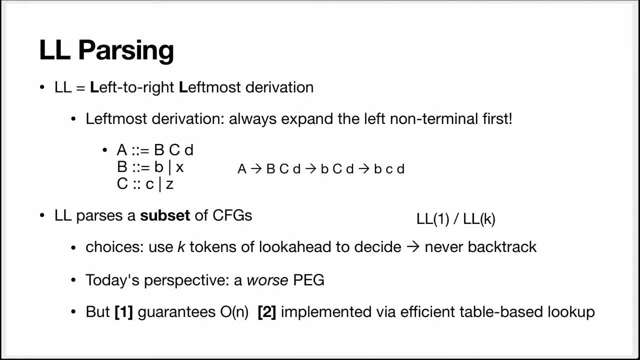 So, LL parsing, what is it? Well, first, what does LL mean? The first L is for left-handed parsing, The second L is for left-to-right, And that's just the direction in which we process the input. There also exists right-to-left parsing algorithms, but they're quite exotic and not often used. 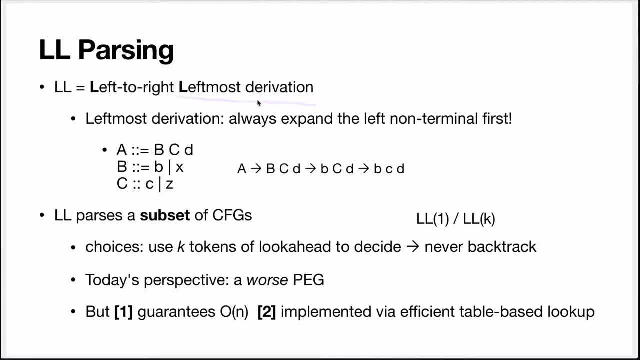 The second L stands for leftmost derivation And derivation here, and derivation here is the kind of derivation that we saw when we were talking about the semantics of CFG. In this context, leftmost derivation means that we are always going to expand the left non-terminal first. 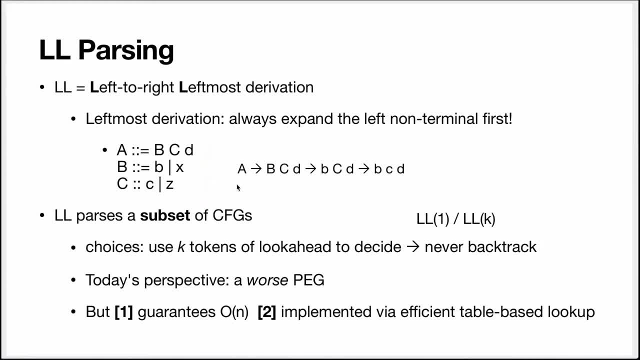 I put a little example here to clarify. You have a grammar And we're going to expand A into its definition, Then we're going to expand capital B into small b And then we're going to expand capital C into small c. This is a leftmost derivation because we expanded B, so the non-terminal on the left before. 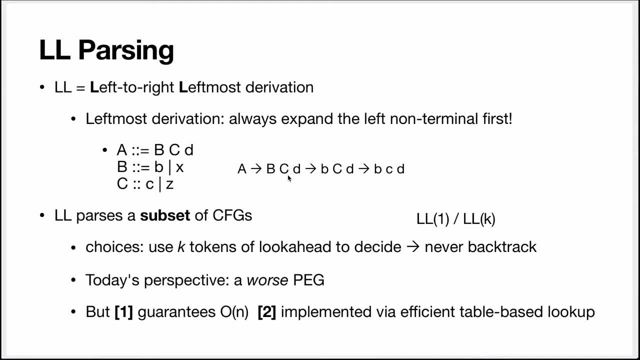 c. At this point you should get a question And the question is okay. But leftmost derivation? Leftmost derivation is something we saw in the context of semantics. It's a way to obtain the language that is defined by the grammar. 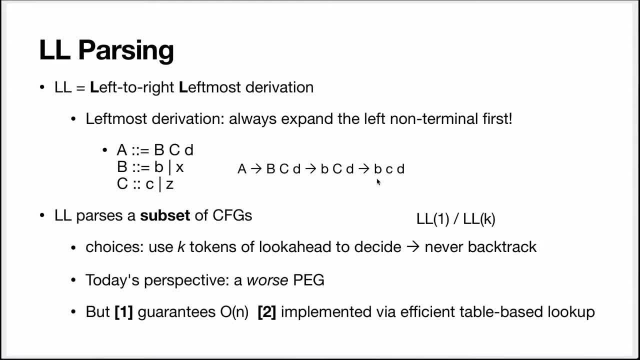 Here we are talking about parsing, And in parsing we always start with the input And we want to see if it matches the language. In this context, what it means to simulate leftmost derivation is that the left non-terminal are going to be matched first. 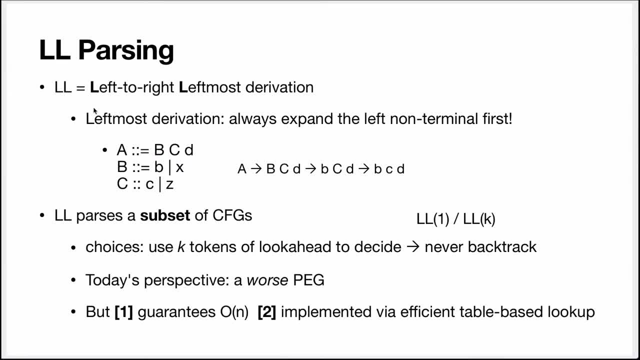 And to understand this I will add some information. The LL parsing algorithm is a top-down recursive descent parser. So just like peg, you can implement them as a set of functions. So say, there's a function to parse A, This function is going to call a function to parse. 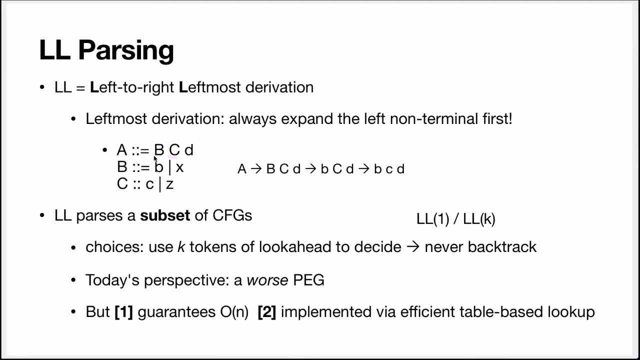 B and a function to parse C, And it will call the function to parse B first. If it calls the function to parse B first, that means that B will be recognized first, which is the same thing as saying that we simulate a leftmost derivation. 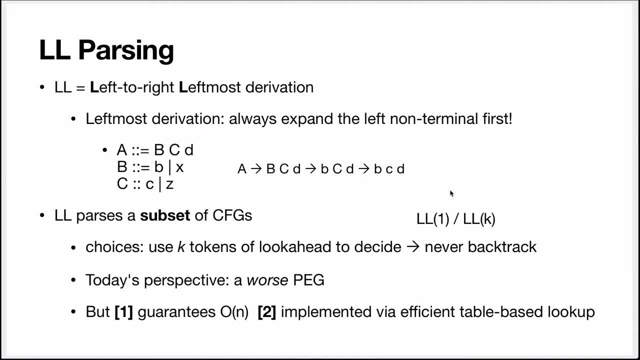 This is all that it means here. So LL parses a subset of context-free grammar. Which subset is that? Well, for this you need to understand how LL handles choices. So remember that a peg parser handles choices by trying every choice alternative in order. 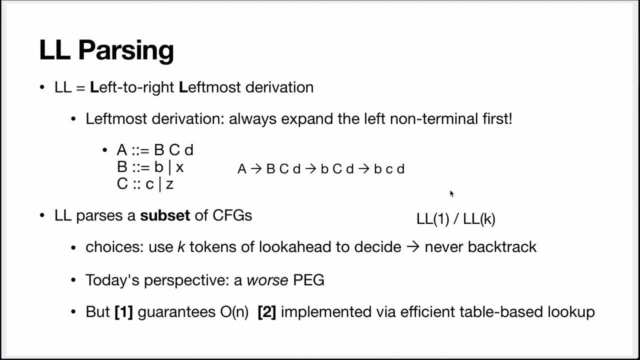 and then picking the first one that match. A LL parser does not even do that. It only picks a single alternative. It only picks a single alternative, And to decide which alternative it will pick, it will use a sort of oracle which is based 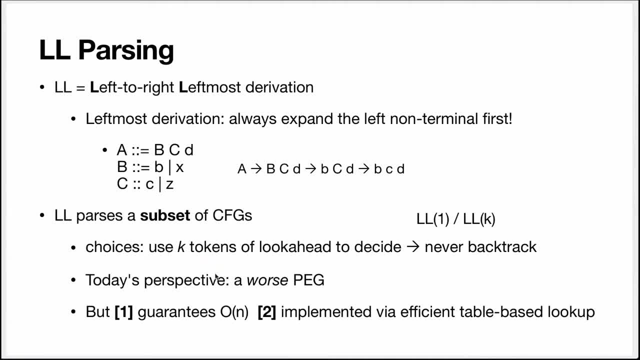 on a look-ahead of K tokens. K is a constant that is decided before you create the parser, And usually K will be 1.. In the rest of the presentation I might assume that it's always 1.. So it looks at this first token and uses that to decide which choice to explore. 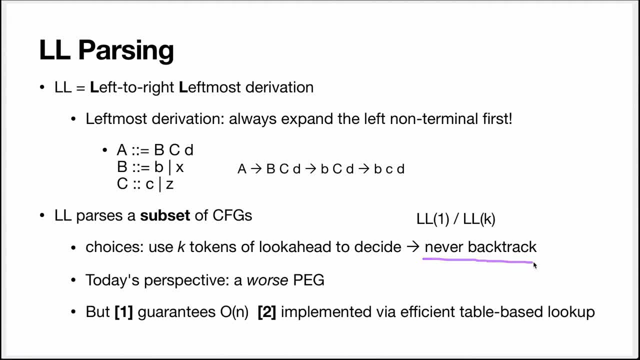 And that causes it to never backtrack. So this is restrictive because it means if you have a choice, all the choice alternatives need to start by a different token. They can never start by the same token, otherwise the LL parsing algorithm cannot decide. 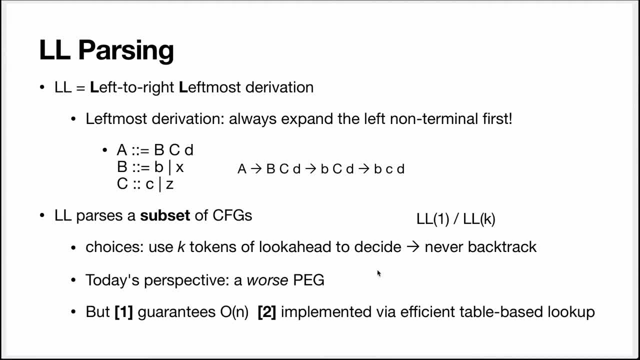 And therefore this grammar will not be a LL grammar. So from today's perspective we can see it's a worse peg. It's strictly worse than a peg because it accepts less languages. The languages for which it's fast a peg will also be fast. 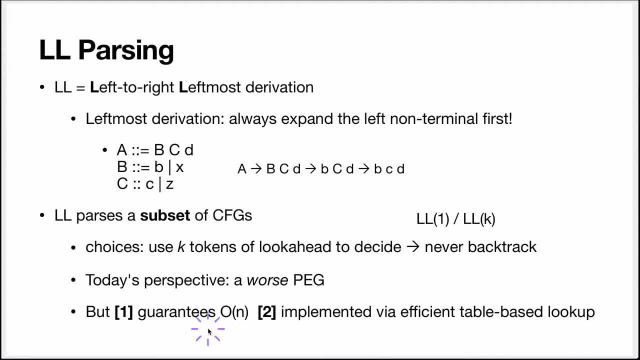 However, it does two things for you. It guarantees that the grammar will be ON. If the grammar is accepted by the LL parsing tool, it means it's ON. That grammar will also be ON peg parser, but the peg parsing tool will also accept grammars. 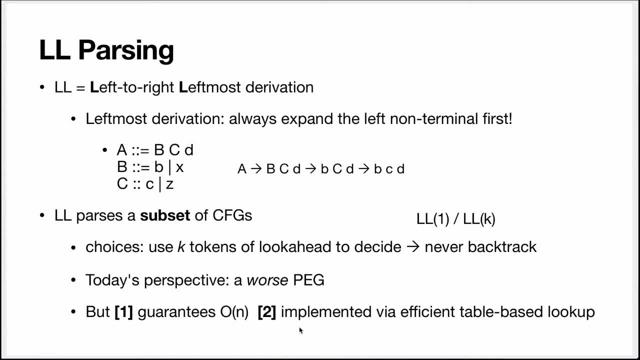 that are not ON. The second thing which is more interesting is that the LL parser can be implemented via a very efficient table-based lookup. So you will take the first token and you use that token to look up in a table which choice alternative you should use. 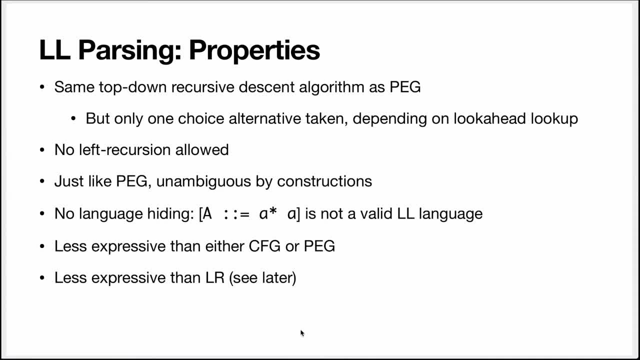 Let's look at some properties of LL parsing. Just like peg parsers, LL parsers are top-down recursive descent parsers. The only difference is that LL parsers are optimized in the sense that they will use the lookahead tokens to decide which choice alternative to use, and so they will not try. 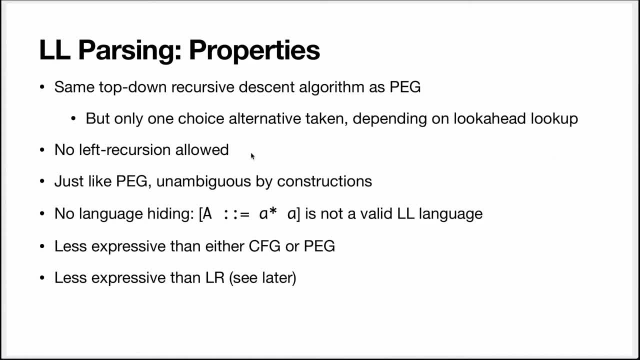 choice alternatives in order. Just like peg parsers, LL parsers cannot handle left recursion because that would cause infinite recursion in the top-down parser. They are unambiguous by construction. Unlike peg, they do not suffer from language hiding, And that's less good than it sounds. 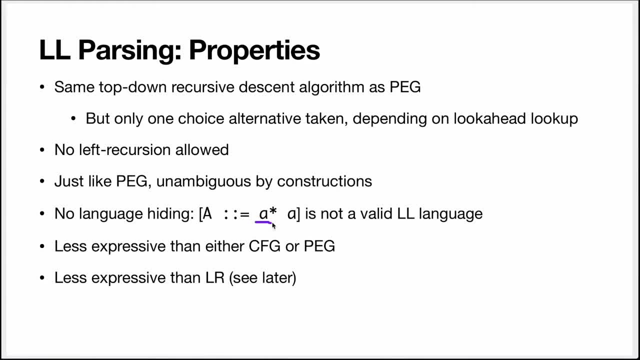 So this grammar has language hiding in peg, because all the a's will be consumed by repetition and there will be no a left for this one here. However, LL does not have this issue, because this grammar is not a LL grammar. The reason why it's not a LL grammar is that LL will not be able to decide whether to repeat. 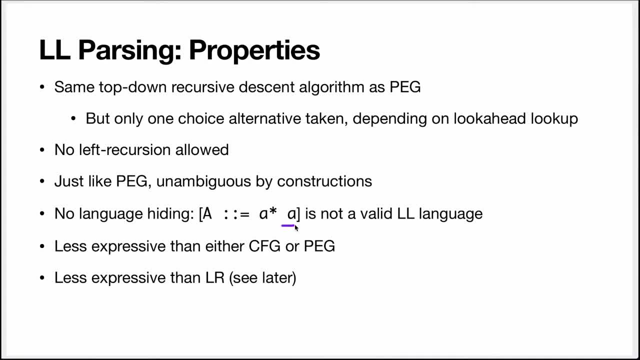 on the a or to just match empty And then match the a to the a. The LL formalism is less expressive than either cfg or peg. In fact it's less expressive than any grammar formalism that we shall see in this course. 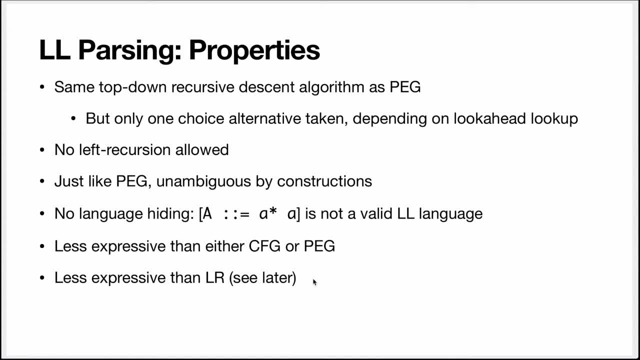 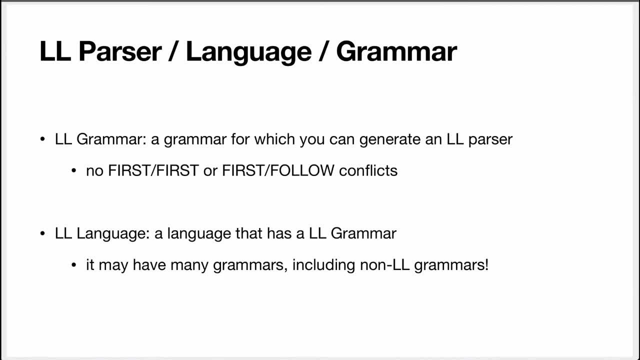 except regular grammars. It is notably less expressive than LR, which we shall see in the next video. So I want to clarify the vocabulary a little bit, because I've been talking about LL, parsers, LL languages, LL grammars. What does it all mean exactly? 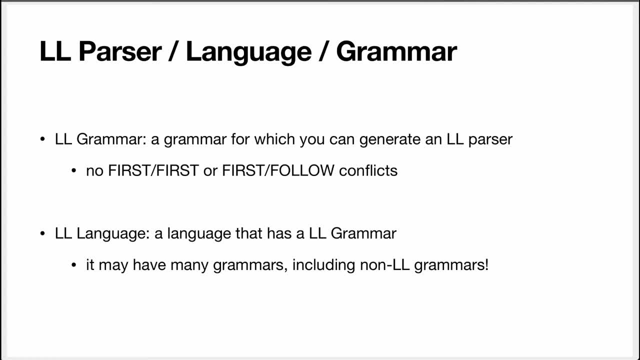 So LL grammar is a grammar for which you can generalize: If you give it to the LL parsing tool, you will not get any first-first or first-follow conflicts. An LL language, on the other hand, is a language that has a LL grammar. 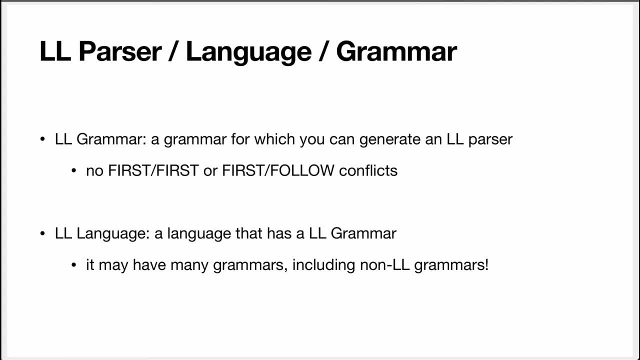 It may have many grammars. in fact, A language is a set of sentences, so there might be multiple grammars that define the same language, And some of these grammars might not be LL grammars. That's fine To be an LL language. it suffices that a LL grammar for the language exists. 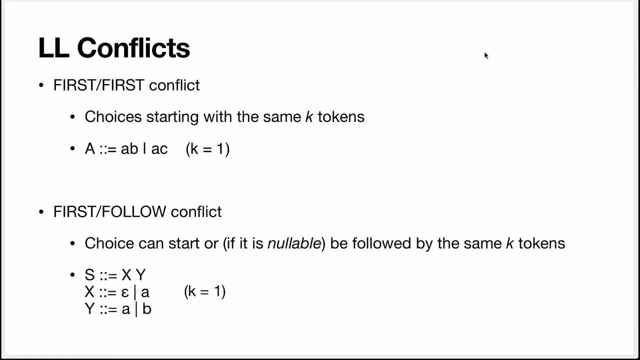 So let's start with LL grammar. So if you feed a grammar to a LL parsing tool, if the grammar is LL, the tool will be very happy and it will generate a parser for you. However, if you feed it a grammar that is not LL, the tool will tell you this grammar. 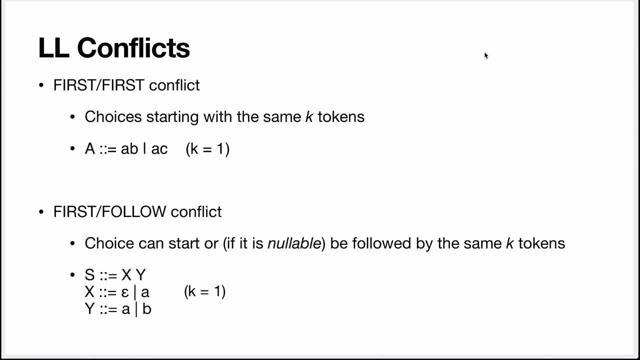 is not LL and it will explain to you why. The way it will explain it to you is that it will give you one of these two messages. So either it will say there is a first-first conflict and a first-first conflict happens when you have a choice. 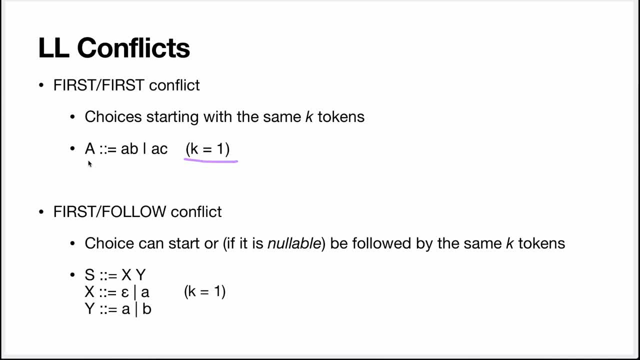 Let's start with the same K token. So here for K equal 1,. this would cause a first-first conflict because both choice alternatives start with A. The other kind of conflict that might be reported is a first-follow conflict. This happens when there are two choice alternatives and one of them can start by a token and 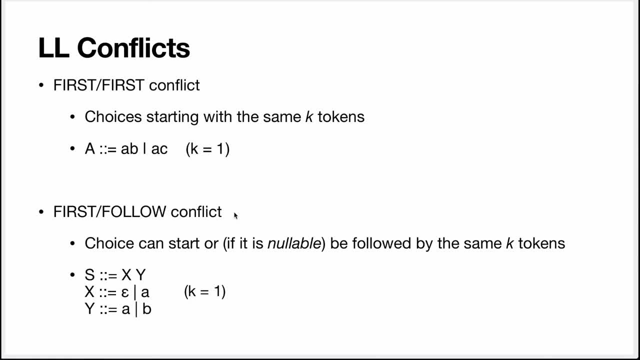 the other one is empty, but the non-terminal can be followed by the same token. This will be easier to understand with an example, So let's start with the same K token. So in this case you see that we have X followed by Y, and X is optional A, so it's either empty. 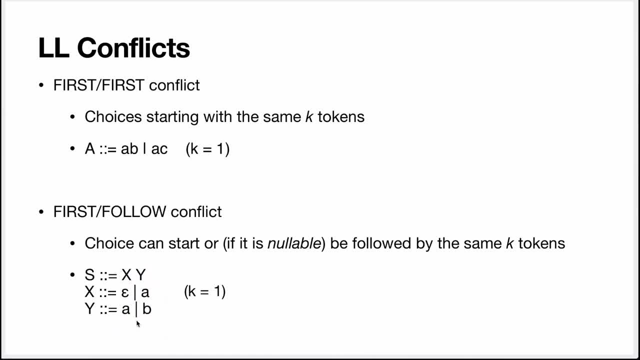 or A And Y is A or B. So say, you are here and you are seeing the token A and of course we are taking K equal 1.. So you're here, you're seeing A. Should the A match X for this alternative, or should? 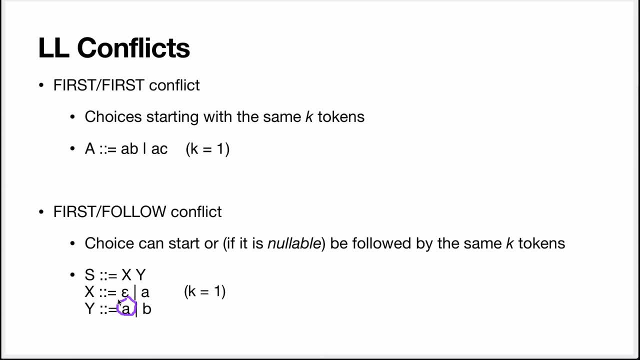 X be matched to empty, And then A Is going to go to Y. Well, the algorithm cannot decide that, and this is a first-follow conflict. So how do we avoid this conflict? We'll focus on first-first conflicts here. 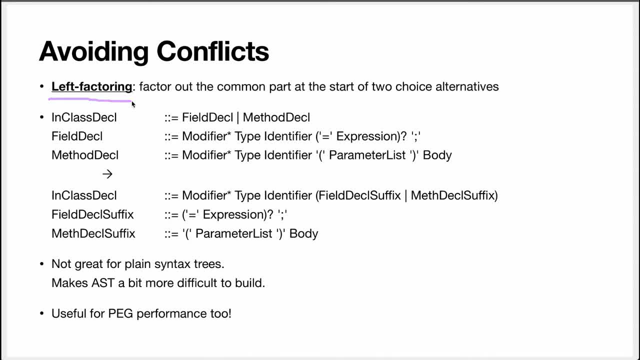 The way we do it is by left-factoring, which is to factor out the common part at the start of two choice alternatives. So here's a very concrete example which is for a java grammar. So you have this in-class declaration rule. 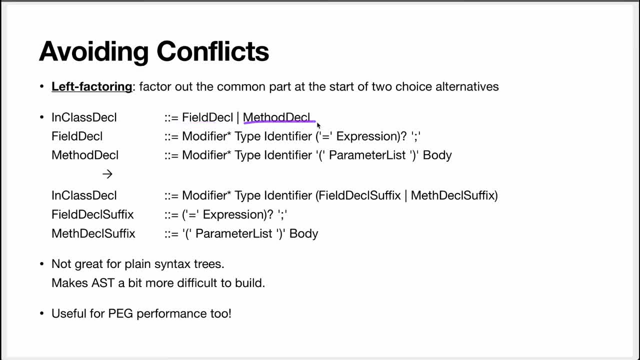 And it defines a choice between field declarations and method declarations. Now, both of these start with the same prefix, which is a bunch of modifiers, so this could be public, final, static, etc. A type for the methods, that's the return type, and an identifier, which is the field. 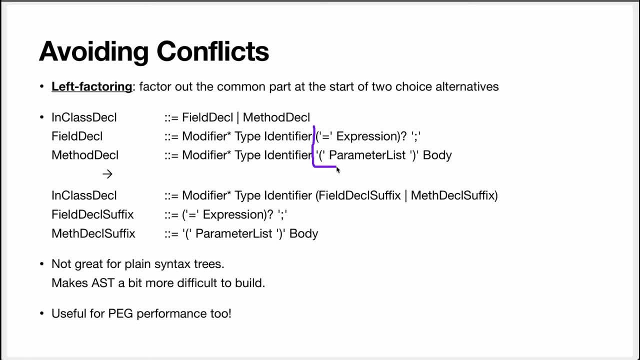 or the method name, And then they have different suffixes here, which are an optional initializer or for the methods, the parameter lists in the body. So what we do is that we extract the suffix. So we extract the suffix And we put it in front of the choice. 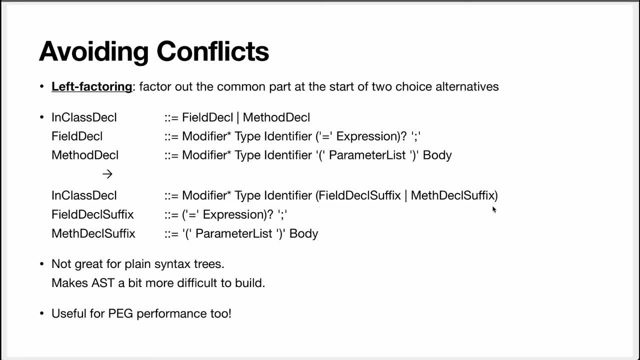 And then we transform the choice, so now that it's a choice between the suffixes. so what's left after we remove the prefix? So this should be simple enough to understand. This is not LL, because both field and method declaration can start by the same prefixes. 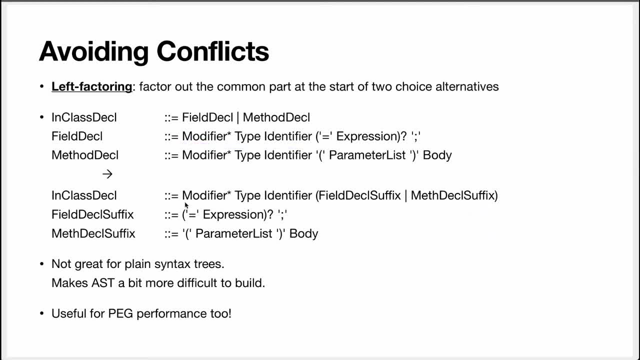 so the same tokens, But this is LL, because now everything is part of the same rule and then only the suffix is different. And it's always going to be different, because here the first token is in open parenthesis, whereas here the first token is either equal or semicolon. 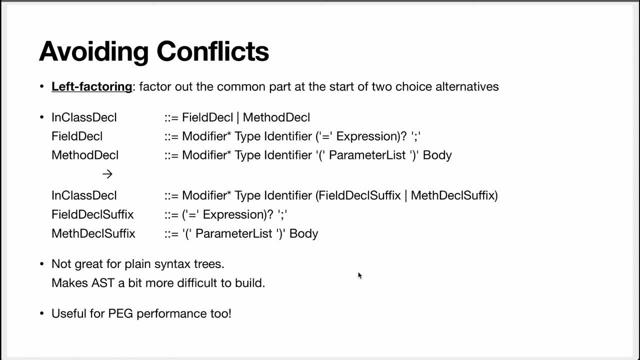 So left factoring is not great if you are using plain syntax trees. Plain syntax trees is when you get a parse tree that follows the rules of the grammar. So in that case you would get actually the prefix and the suffix coded into your tree. 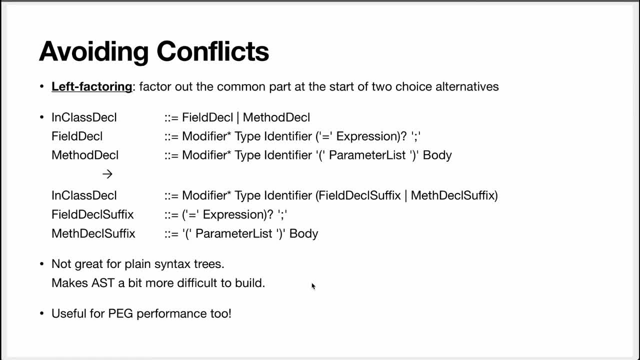 It also makes it a bit harder to build the abstract syntax tree, but that depends on the tool that you are using and how it works to build syntax trees, so it's hard to comment. in general, Left factoring can also be useful for peg performance. 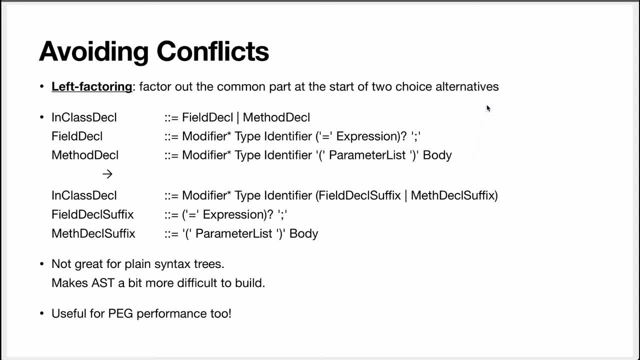 This will work in peg, but it will cause duplicated work. sometimes Say you are trying to parse a method. well, first you have to try to parse a field, which means you have to parse the whole prefix Before noticing that, Oh, actually it's a paren, so it's not a field declaration. 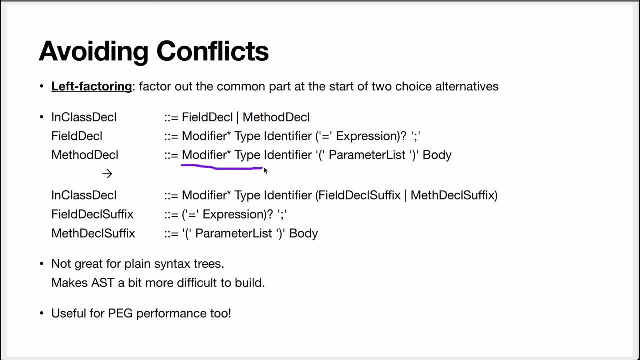 So then you need to backtrack, try the method declaration and reparse the whole prefix again. So you're wasting work, basically, And in this case it might be useful to left factor to improve peg performance. Here's a question that you might have. 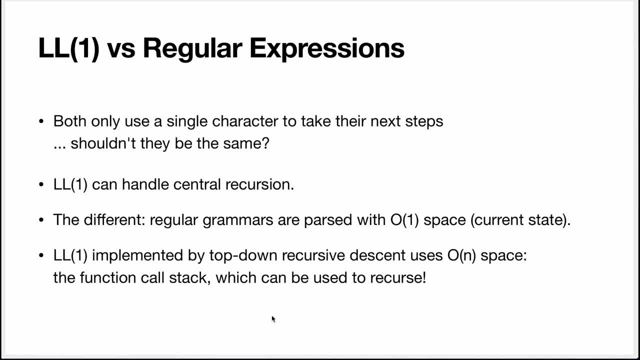 We've seen that LL parsers only look at a single character, or I should say, symbol or token, And depending on that, They take the next step. So isn't that exactly what we did for regular expressions with deterministic finite automaton? And the answer is no. it's not quite the same. 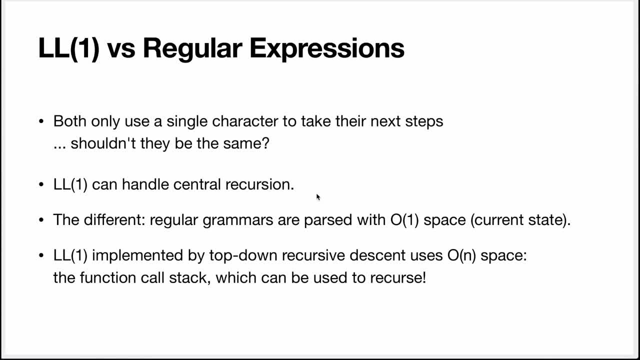 And in fact LL grammars, they can handle central recursion. So remember the examples. with the nested parentheses, The difference is that regular grammars, they are parsed with O space. So the only piece of memory that you have in a deterministic, finite automaton. 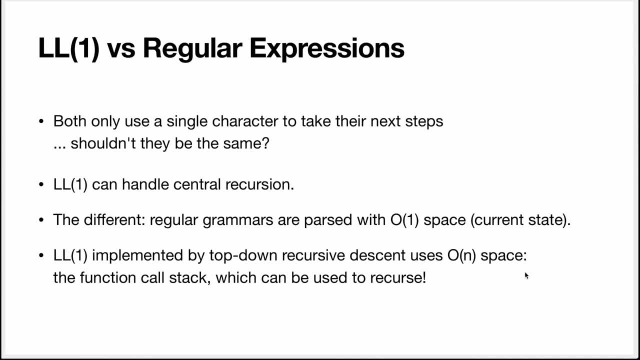 Is the current state in the automaton. LL, on the other hand, is implemented by top-down recursive descent, And so it uses O space and the N space. here is the call stack, And this is the extra memory that we need to recurse and to implement central recursion. 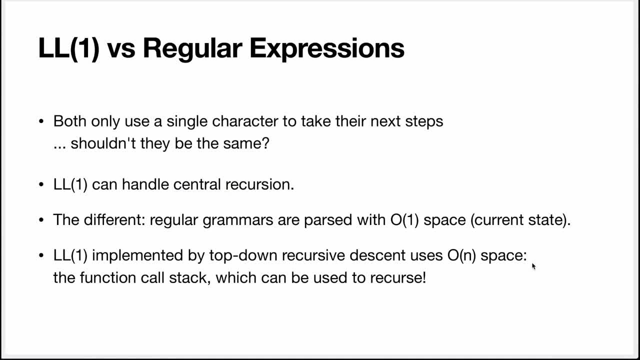 It's also rated. Remember that context-free grammar can be parsed with the NDPDA, so a non-deterministic push-down automaton. Actually LL grammar can be parsed with a NDPDA. It's also rated. Remember that context-free grammar can be parsed with a NDPDA. 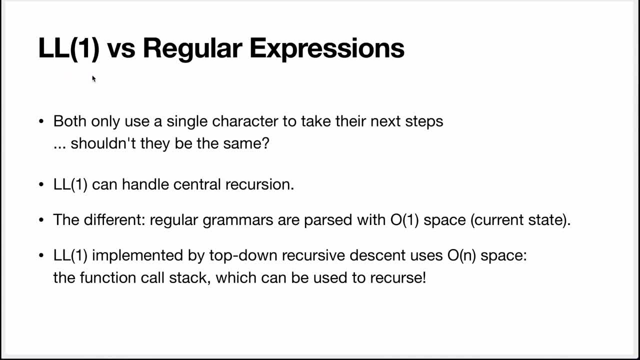 It's also rated. Remember that context-free grammar can be parsed with a deterministic push-down automaton, And so a deterministic push-down automaton is just like a finite automaton, but it also has a stack that it can use, And the stack again, that's the O space.